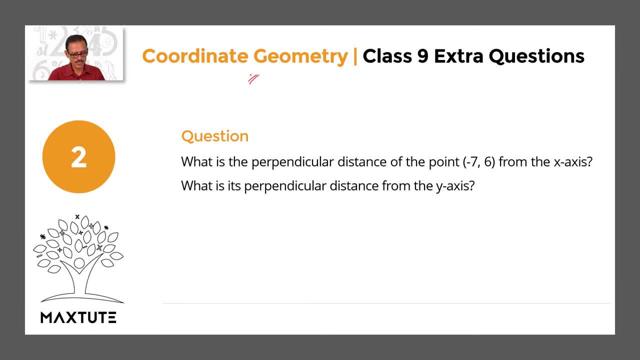 CBSE class 9 math extra practice question. This is from the chapter coordinate geometry. This question is an easy question conceptually, but there's a small trap in the way it is worded. So read the question carefully and then answer it properly. Let's get started. Let's have a look at 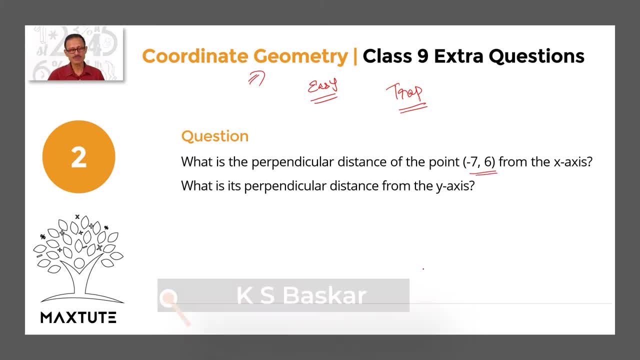 the question: What is the perpendicular distance of the point minus 7 comma 6 from the x-axis? That's part one of the question. The second part to it: what is its perpendicular distance from the y-axis? Some of you, as you read it, will want to, will be raring to go and want to give an answer. 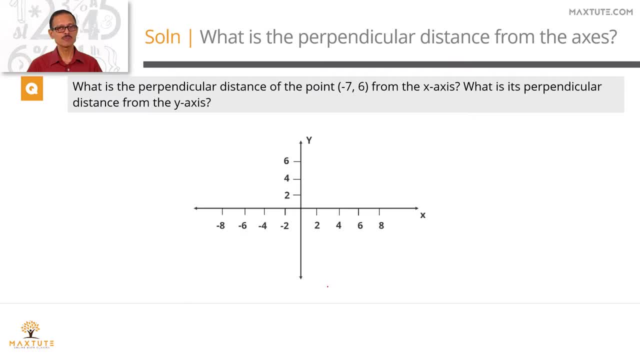 to this. Just hold on for a minute. We'll first plot this point and then look at what could have been the answer and what is the answer, Looking at this point, whose coordinates are minus 7 comma 6.. We're talking about x-axis. The x-coordinate is minus 7.. Minus 7 is a point that lies in between. 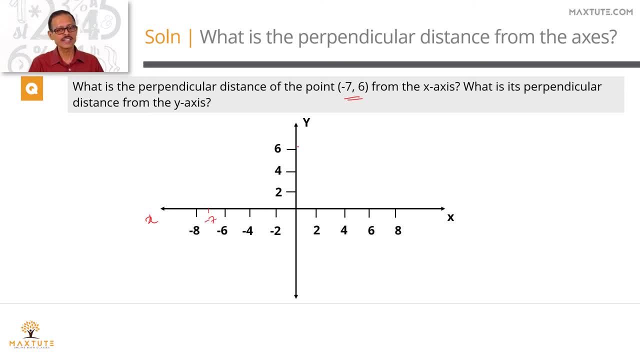 minus 6 and minus 8.. So this is minus 7.. Its y-coordinate is equal to 6,, which is this: So let's draw lines parallel to y-axis from minus 7 and parallel to x-axis from 6.. So the point. 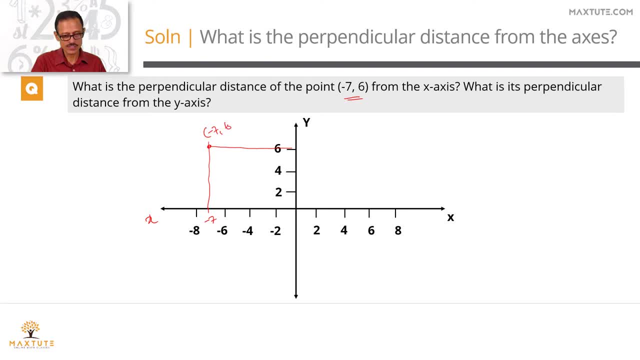 where these two lines cut is going to be the point of this. So this point minus 7, comma 6 lies at this place. What is the first question? What is the perpendicular distance of this point from the x-axis? So obviously we're going to be. 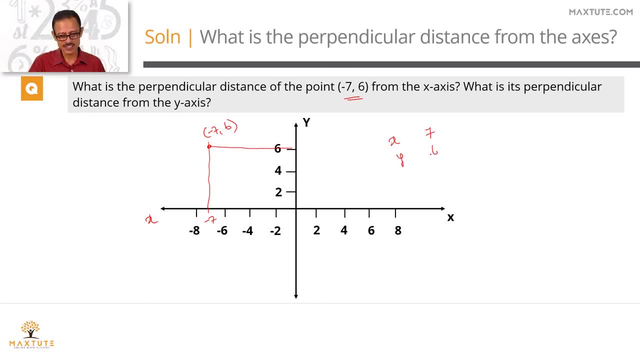 jumping and saying that it is 7 units from the x-axis and it is 6 units from the y-axis, which is essentially the magnitude of the x and y-coordinate. But hold on. Let's start with the first question slowly and check whether this is the answer. This is the answer which it appears. 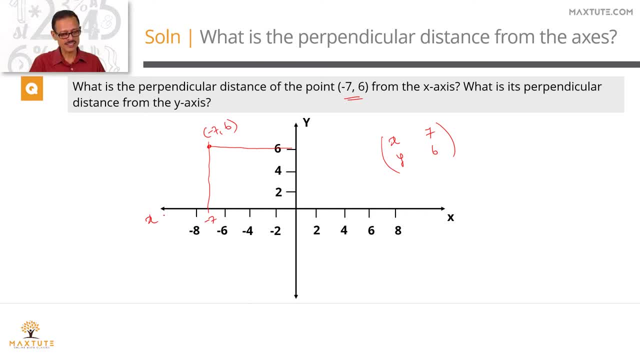 to be for us. We're looking at the perpendicular distance from the x-axis. The horizontal axis is the x-axis. Perpendicular distance of this point from the x-axis: How much is it? It's actually 6 units, which is nothing but the y-coordinate, The perpendicular distance of the point from the 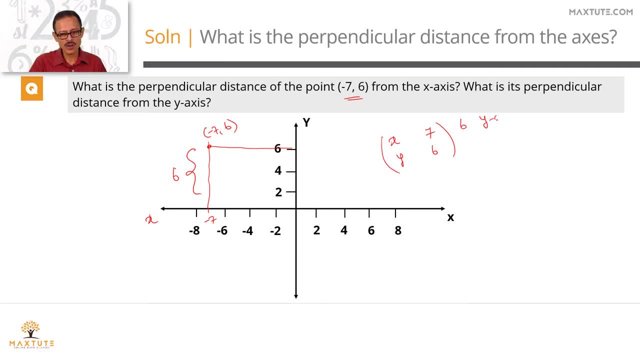 x-axis is actually measured using the y-coordinate of that point. So it's actually 6 units and it is not 7.. What's the second question? What is the distance from the y-axis? The vertical axis is the y-axis. What is the perpendicular distance of this point from the y-axis? This: